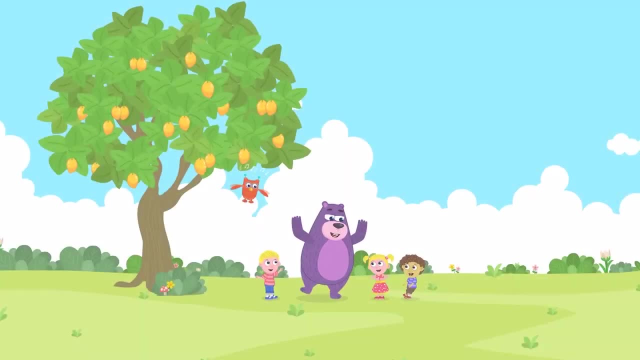 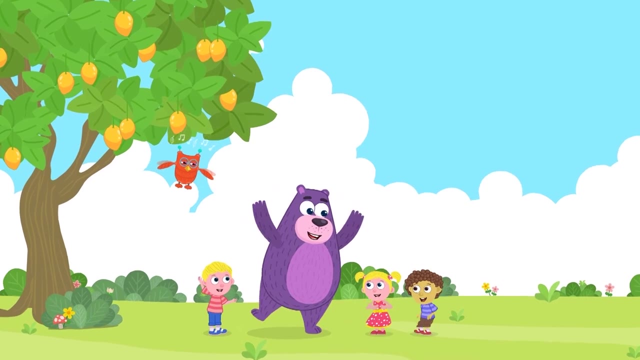 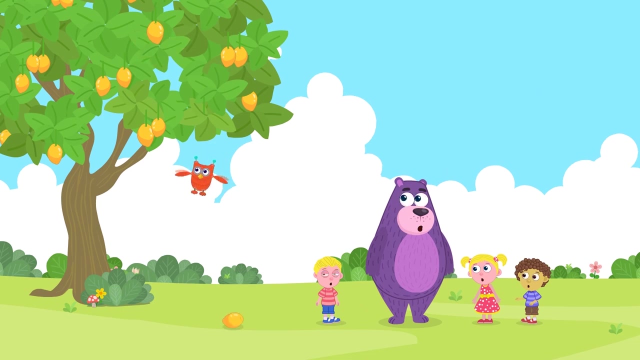 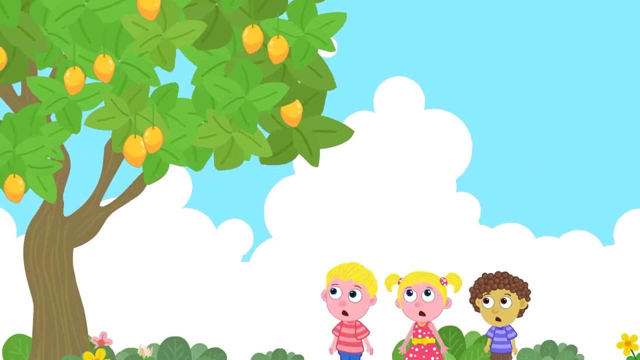 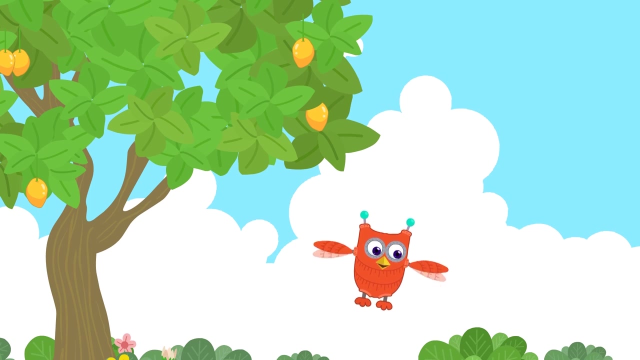 Polly Olly. It's such a beautiful day, Polly Olly, Lily and Jack are playing and dancing. Hey, Olly, Are you okay? Yes, I guess I am fine now. Phew, Thank goodness you're okay, Olly. 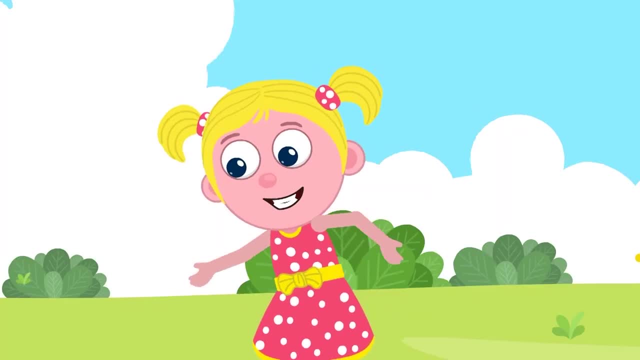 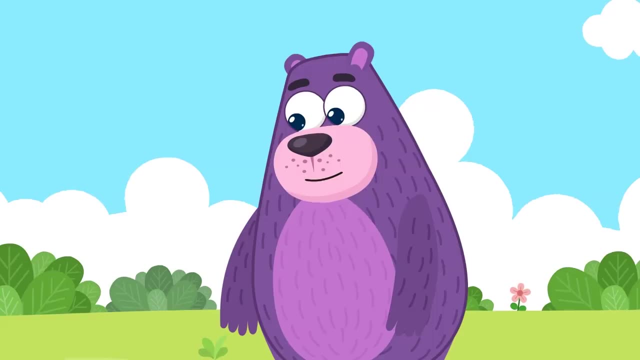 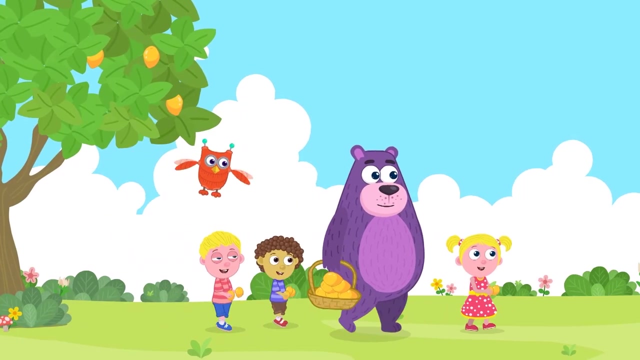 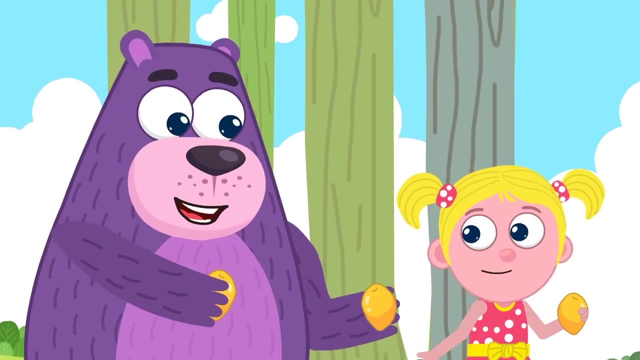 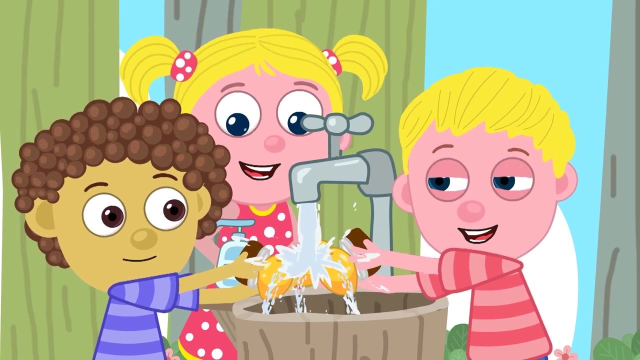 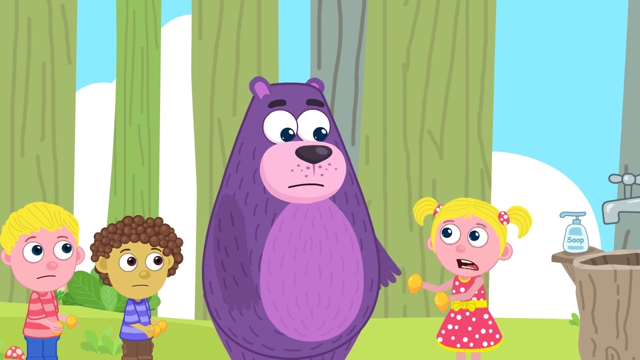 Wow, So many mangoes. Ew, They're all sticky. Look at my hands. Don't worry, We can go wash our hands and the mangoes at my house. Hey, Polly, What did you do that for? I haven't finished. 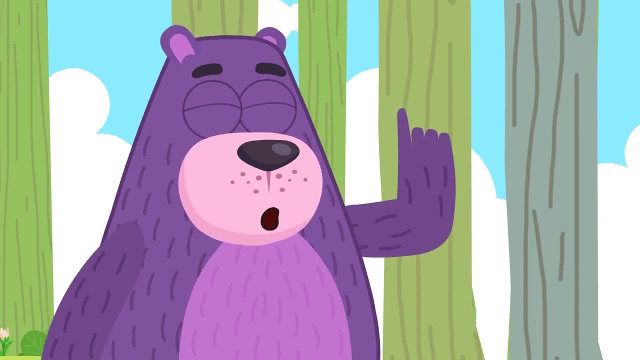 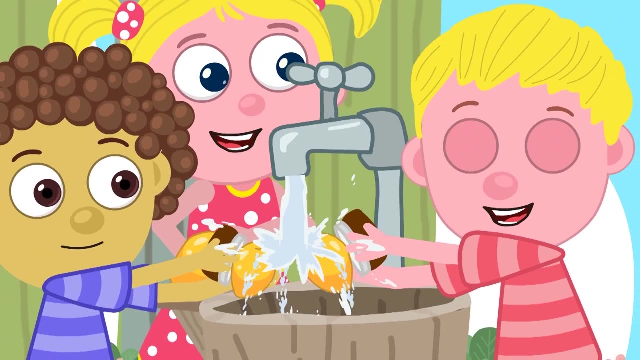 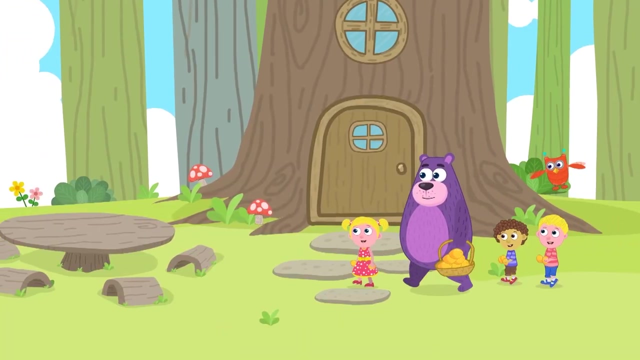 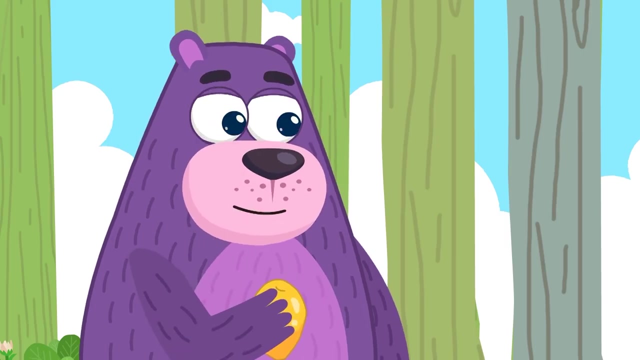 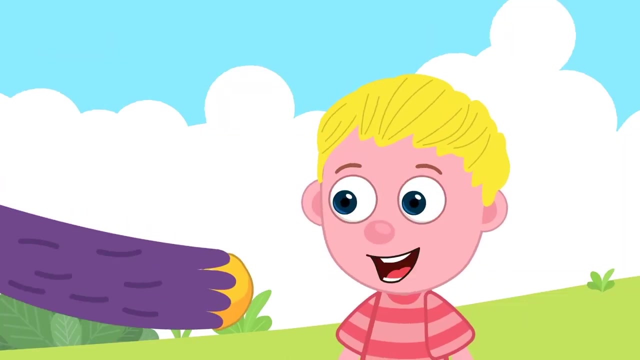 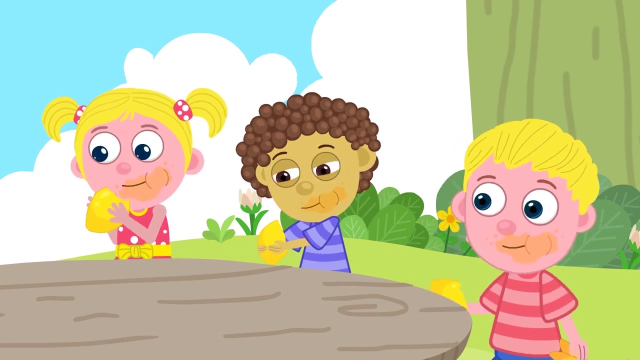 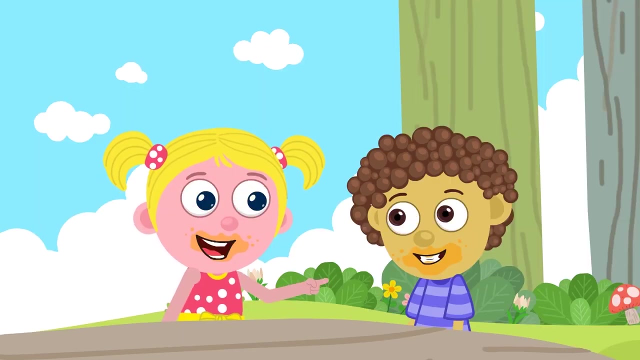 We don't need any water while we're scrubbing and it's important not to waste clean water Ready to rinse. Okay, Time to eat. Here you go. Try eating that without getting messy. Mmm, That was delicious. You've got mangoes stuck between your teeth. You look funny. 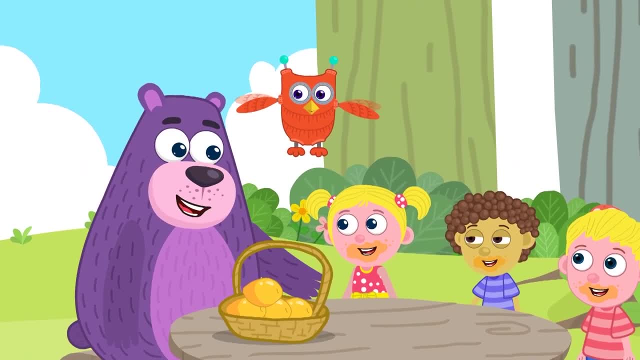 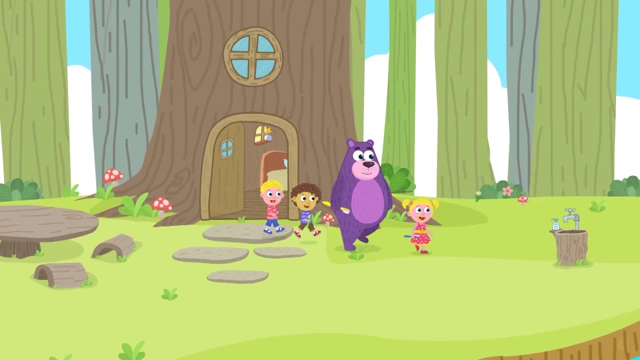 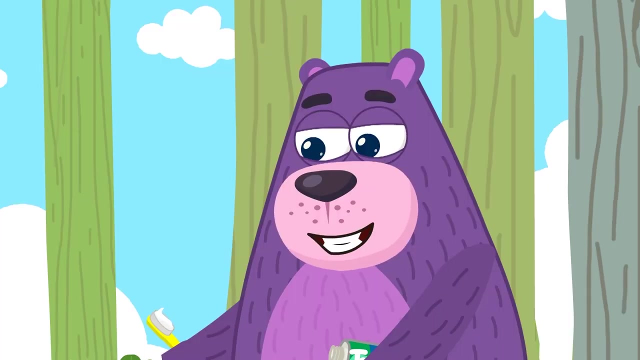 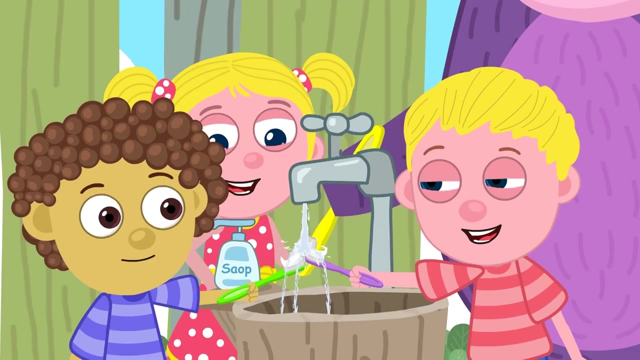 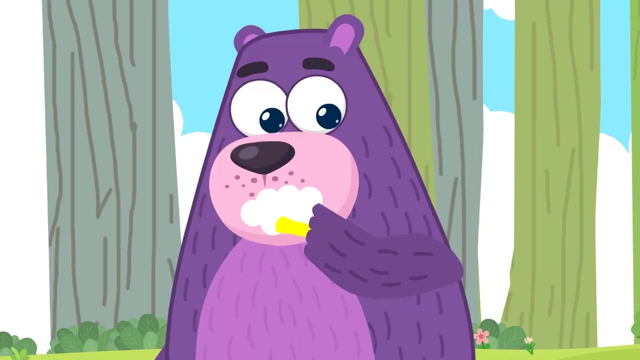 So have you? Come on, We better go and brush our teeth. Are we saving water again? Yes, Olly Polly, turn off the water. What The water? What, Oh The water? Well done, kids. It's not always easy to remember to save water. Sometimes we have to remind each other. Keep up the good work.